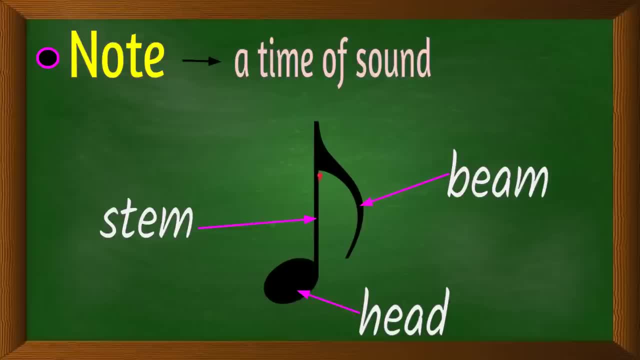 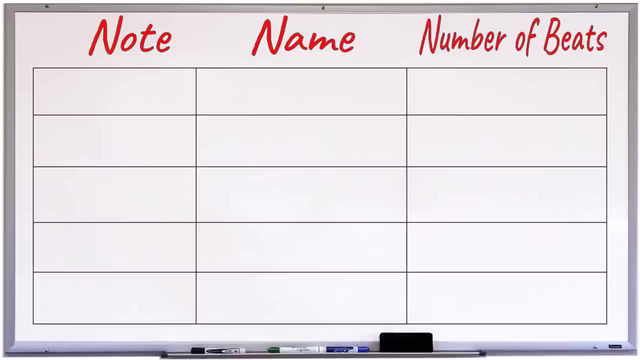 This is the head, This is the stem And this is the beam or flag. Now let's go to the note symbol itself: the name of that note and the number of beats. Each note has a value of time. The number of beats tell how long a note is played or sounded. 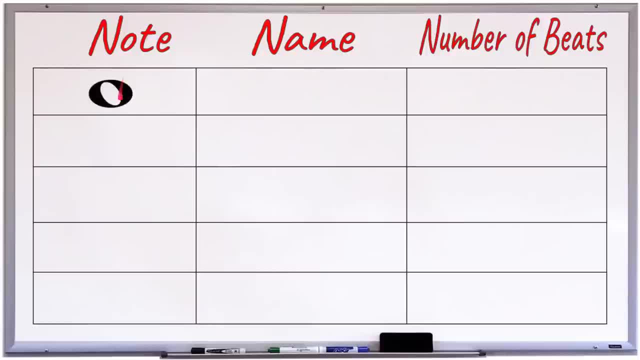 Amazing, Let's proceed. Okay, for this one. it's the head only. It's called a whole note And it has four beats. This one: it has a head, not shaded or unshaded head, with a stem already. 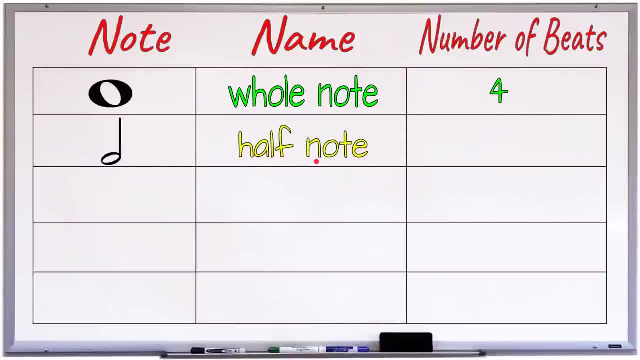 This is what we called a half note And it receives two beats. This one is the head is already shaded and it has a stem. It's called a quarter note and it receives one beat. Next for this one: it has already a beam here or a flag. 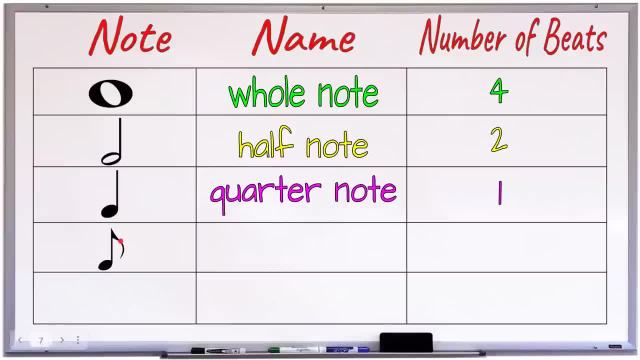 Next for this one. it has already a beam here or a flag. Next for this one: it has already a beam here or a flag. Only one flag or beam. It's called eighth note And it receives one half beat. 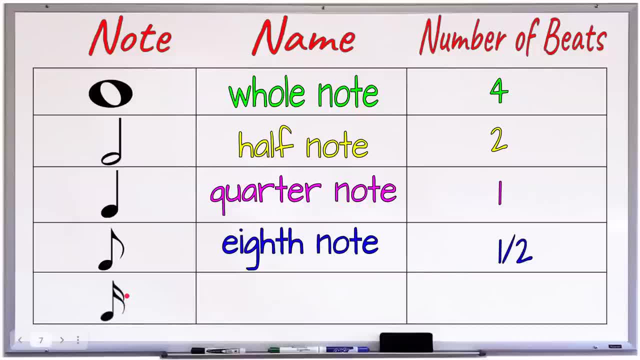 For this one we have two beams or two flags already. It's called sixteenth note And it contains one fourth beat. Again, this is a whole note. For this one, it has a head. It has four beats. Next for this one: it has a head. 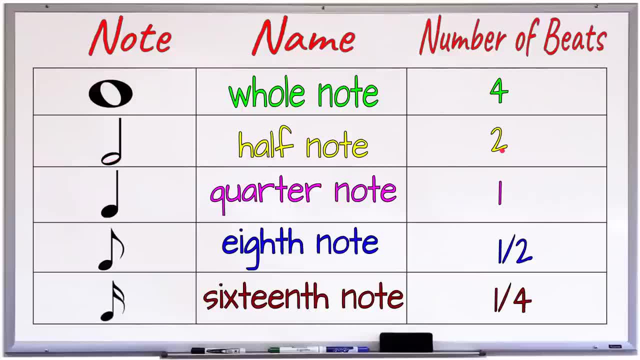 Again, this is a whole note. Again, this is a whole note. this one: this is a half note. It has two beats. This one is a quarter note. It has one beat For this one. it has a flag already. Eighth note and it has one half beat For. 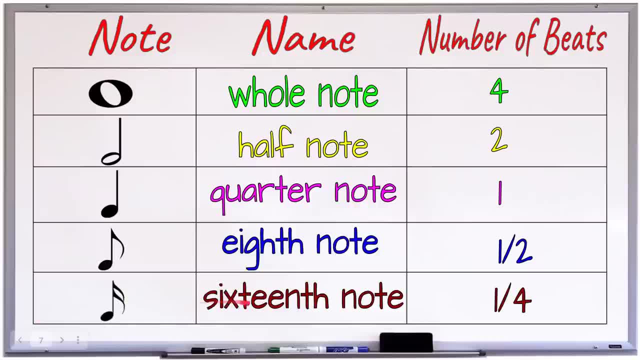 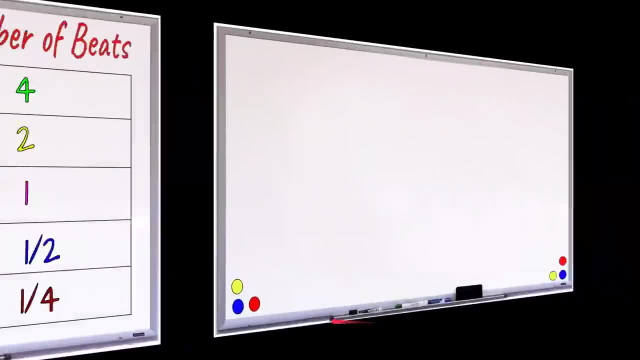 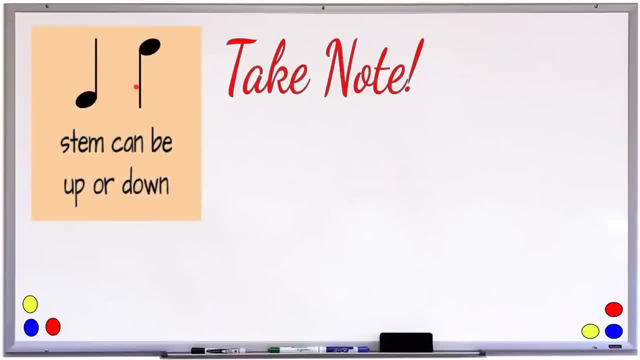 this one. it already has two flags or two beats. It's called sixteenth note and it has one fourth beat. Let's proceed. Take note that the stem of a note can be up or down. The stem that is up and down doesn't affect the value or the number of beats of. 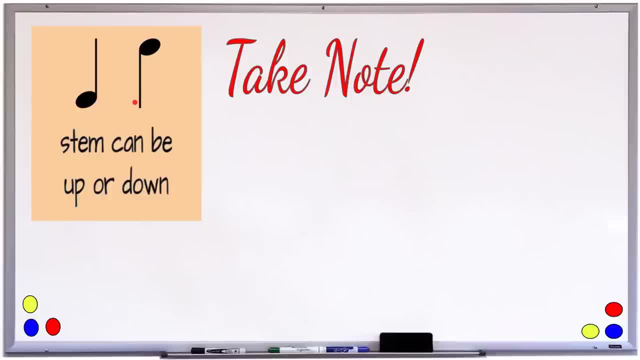 that note, And also for the beam or the flag itself. it's always pointed at the right side of it. Next, let's proceed. These are called two eighth notes that are beamed together, So they are put together. That's why they are called notes that are beamed together For. 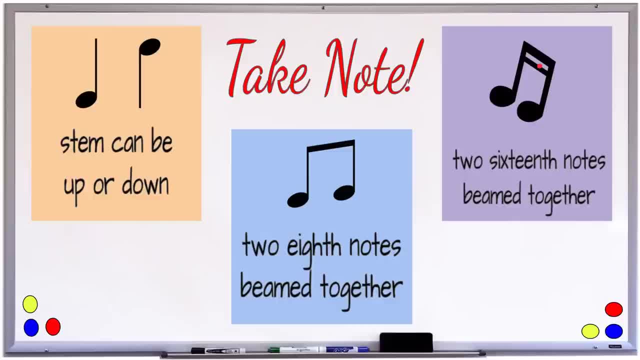 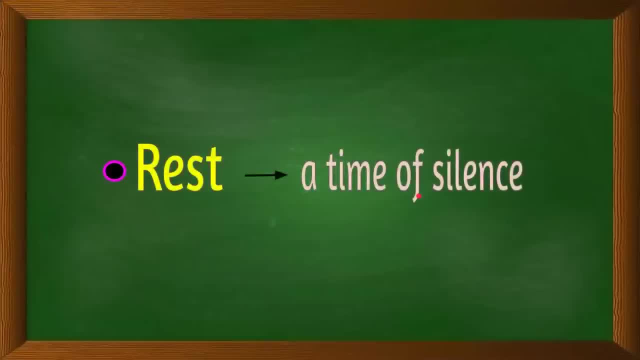 this one. they are two sixteenth notes that are beamed together. They are put together. Okay, Let's proceed to our rest. Rest is the time of silence. So there is no sound at all. You're not making a sound, And that is called rest. It's time of silence, Okay, So let's go to 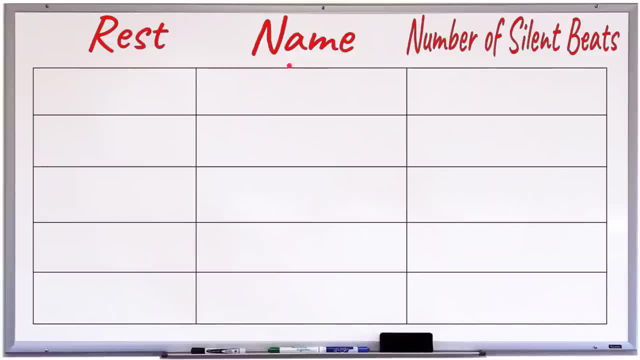 our rest symbol, the name of that rest and the number of silent beats. This time it's four silent beats already. Okay, Let's go to this one. It's like a box that is hanged down below the line, Or simply what we call a rectangle facing downward. That's called 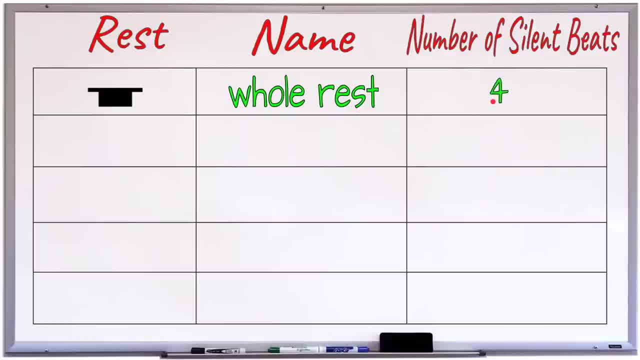 a whole rest And it receives four silent beats. It has four silent beats, Whole rest, Four silent beats. For this one it's the opposite of the first one. It's a note that's going to be played Now. this is the second half. Now the first half is going to have. 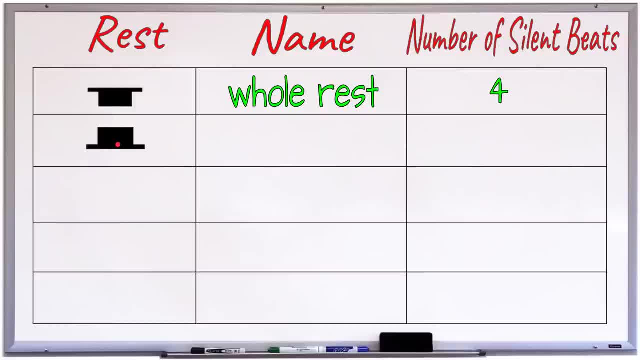 a little bit more of a cut, And so the next half is going to be played. And now the next half is going to be played, And so the next half is going to be played. Now this is going: its box is facing upward, or the rectangle is facing upward and it's 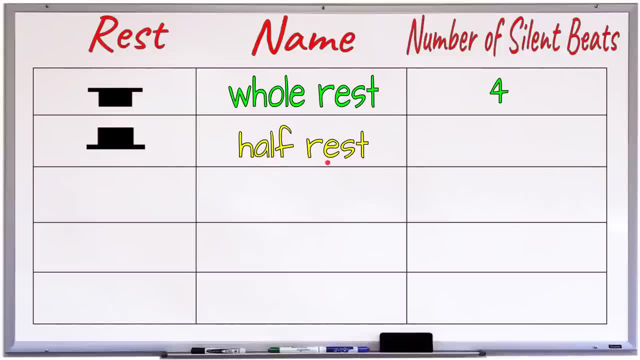 called a half rest, again half rest. it receives two silent beats. it has two silent beats. okay. next this one. it looks like a crooked letter Z to me and it's called quarter rest. again quarter rest. it has one silent beat. only for this one. it looks like number seven. this is the flag: one flag or one beam. it's called a. 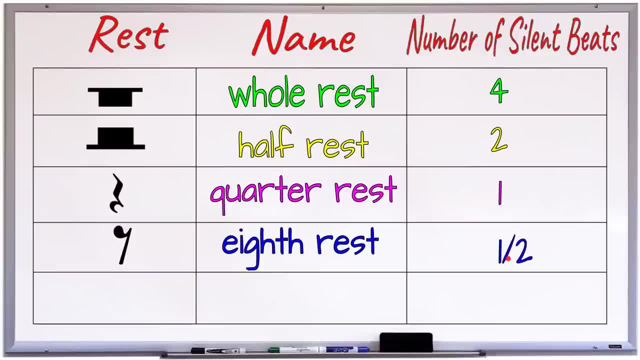 thrust okay, and it has one half silent beat for this one. it has two flag already. it's cold. sixteenth rest and it has 1, 4 feet 1. fourth silent beats. again. that's named. again, this is hole rest. it has four silent beats. this one half rest it has. 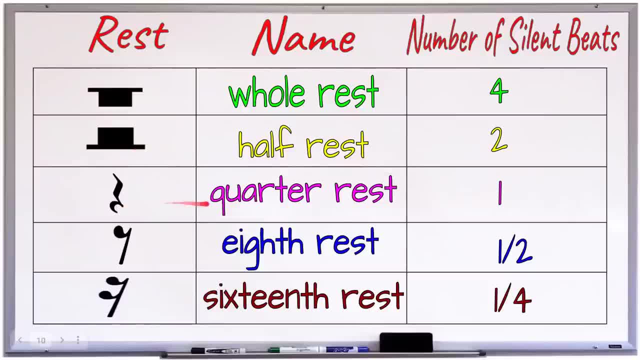 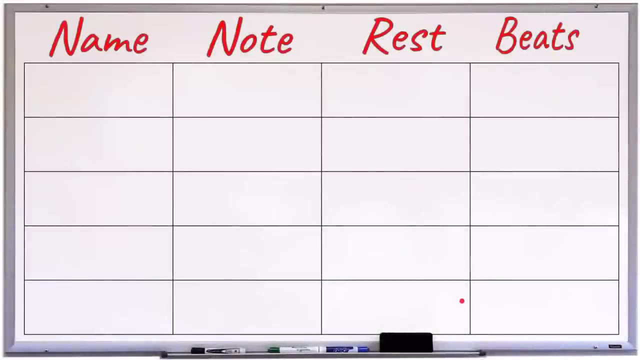 two silent beats. this is a quarter rest and it has one silent beat. this is an eighth rest. One half silent beats For this one. it's a sixteenth rest. It has one-fourth silent beats. Okay, let's proceed to our summary. 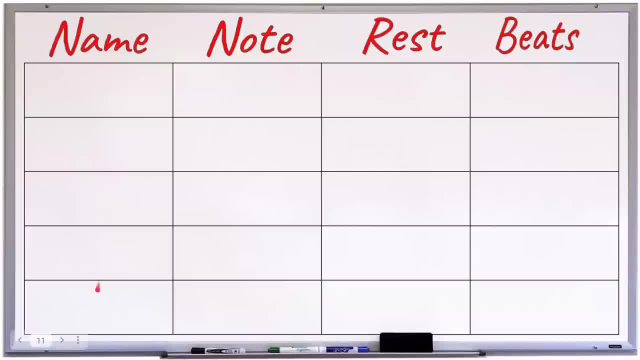 Okay, so there is a symbol here, the name, and then the note, the rest and the beats. Okay, all right. So this is the whole note, whole note. okay, Again, whole note, the head, and then this is a whole rest. 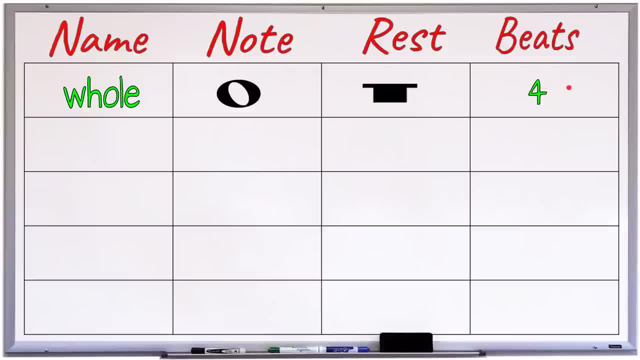 They both receive four beats. It's that the note has a sound and for the rest it has no sound, But they have the same beat four. Okay, next let's go to half. This is half note. This is half rest. 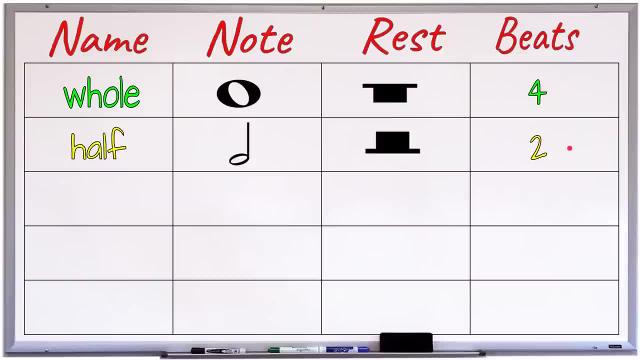 They both have two beats, Or the time value, they have two, The note has two and then the rest also, they have two. Okay, next we have quarter Quarter note and the quarter rest. They both have one beat, okay. 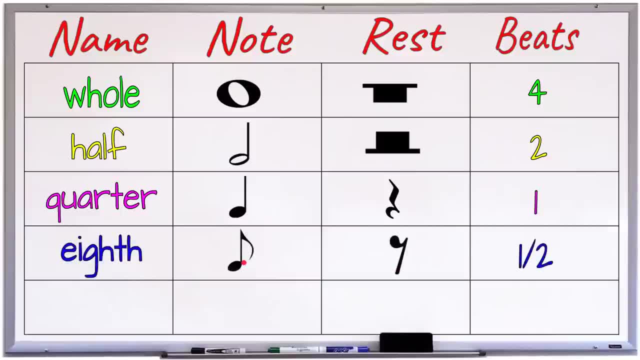 Next we have eighth note. This is the eighth note and this is the eighth rest. They both have one half beat, okay. Next we have sixteenth note. This is the sixteenth note, This is the sixteenth rest, And both of them they have one fourth beat. 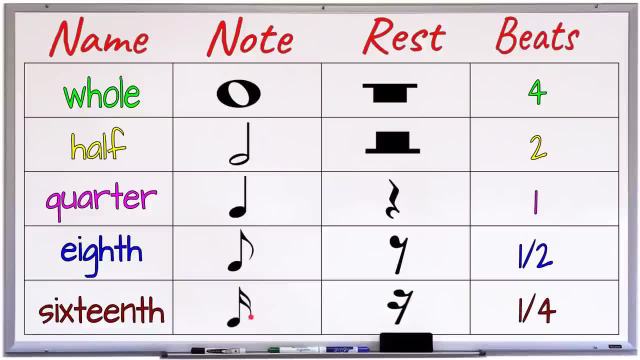 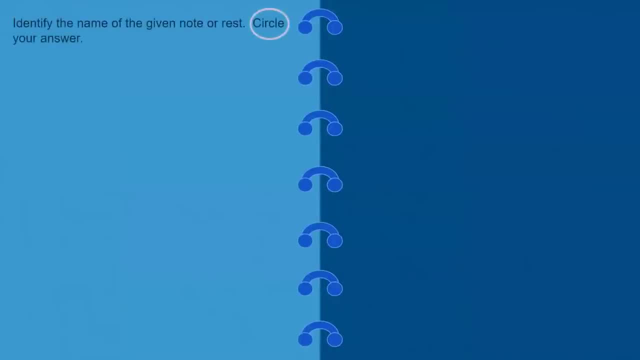 Again, for the notes: here they have sound. For the rest, here they have silence or no sound at all. Okay, That's why it's called rest. Okay, now let's go to our activity. Okay, we're going to name the given note or rest. 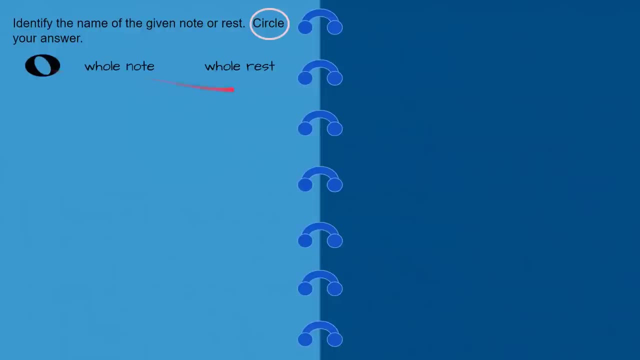 Okay, for this. one whole note or whole rest, Correct, This is a whole note. Next, this is half note or quarter note. Correct, It's quarter note. Okay, for this one. it has two notes. It has two beams or two flags. 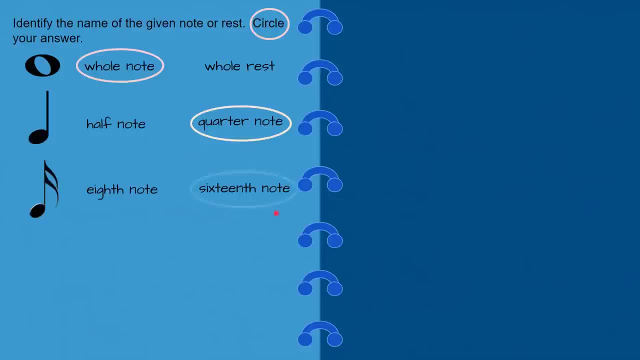 Okay, Eighth note or sixteenth note- Correct, It's sixteenth note, This one, okay, its head is not shaded at all. Okay, half note or quarter note- Correct, It's half note For this one. it has only one flag or one beam only. 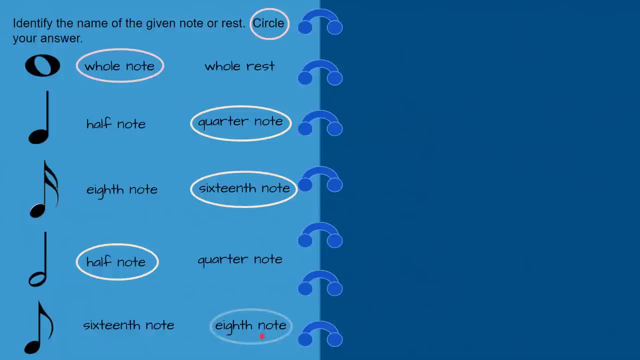 Sixteenth note or eighth note? Correct, It's eighth note. Okay, here, this one. It's facing upward Half rest or whole rest? Correct, It's half rest, This one. it has only one flag or one beam. 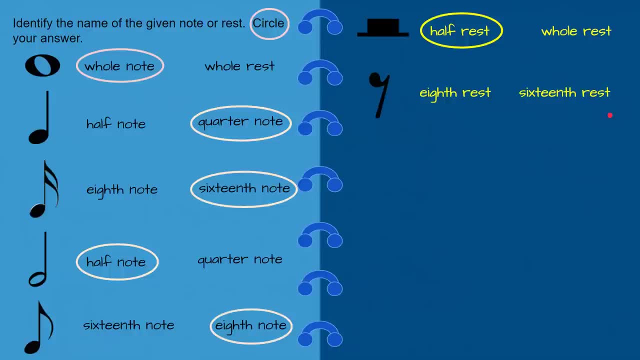 Okay, Eighth rest or sixteenth rest? Correct, It's eighth rest For this one. two flags already. Eighth rest or sixteenth rest? Correct, It's sixteenth rest For this one, This one. This is Quarter rest, or eighth rest? 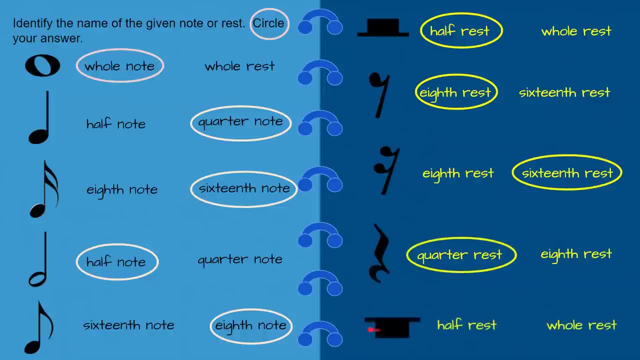 Correct, It's quarter rest. This one is facing downward Half rest or whole rest. Correct, It's whole rest. Very good, Let's review. This is Whole note. This one shaded head Quarter note. Correct This one. 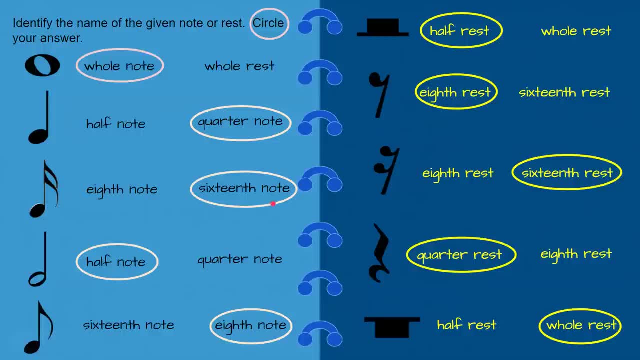 Two flags. Sixteenth note: Correct, Okay, Correct, This one is unshaded. a shaded head? half node: Okay, This one. only one flag or one beam. eighth node: Correct For this one. facing upward half rest, This one. eighth. 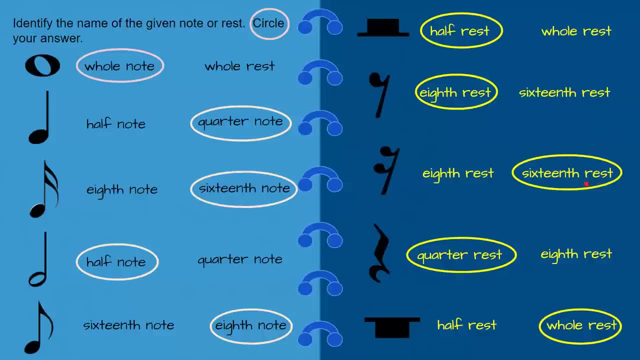 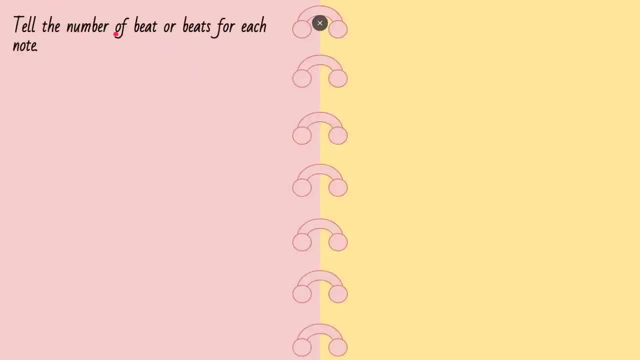 rest. Okay, For this one, this is called sixteenth rest. This is a quarter rest, And for the one facing down, that's whole rest. Okay, Let's proceed to our next one. We're going to tell the number of beats, or beats, for each node. Okay, This is a whole node. This is. 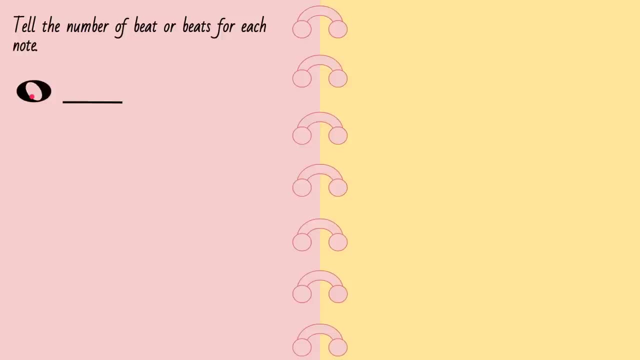 only the head. How many beats Correct? It's four For this. one shaded head already. This is we called quarter node. Okay, It has one beat Correct For this one. it has a one beam already, One flag. That is an eighth node. How many? 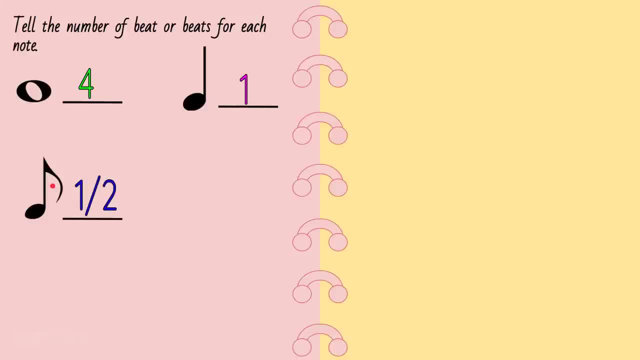 beats Correct. It has one half One half beat. This is unshaded head, So it's okay, it's half node. How many beats Correct? Two. Okay For this one. two flags already. This is called. 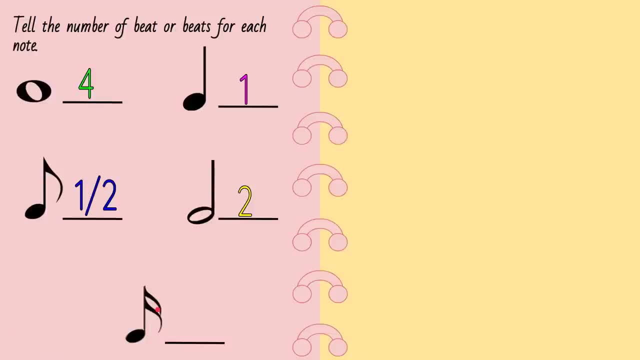 sixteenth node: How many beats Correct One? fourth, Very good, Let's proceed to our silent beats of rest. This one, this is what we called a quarter rest. Correct Quarter rest. How many beats does quarter rest has? Correct One, How about this one? Two flags, So it is sixteenth rest. Sixteenth. 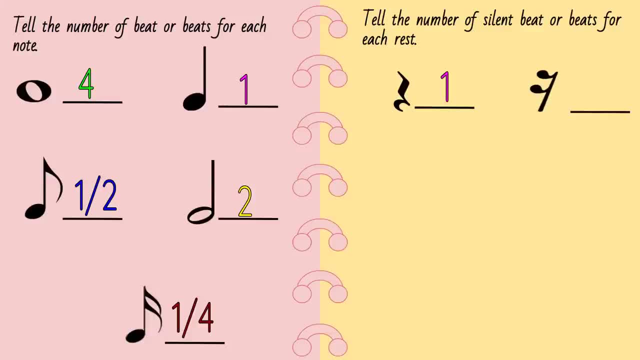 rest How many beats or silent beats? Correct: One, fourth only. Okay, This one. this is eighth. rest Only one flag. How many beats, Or how many silent beats? Correct: One half silent beat. Okay For this one. this is a whole. rest The box. 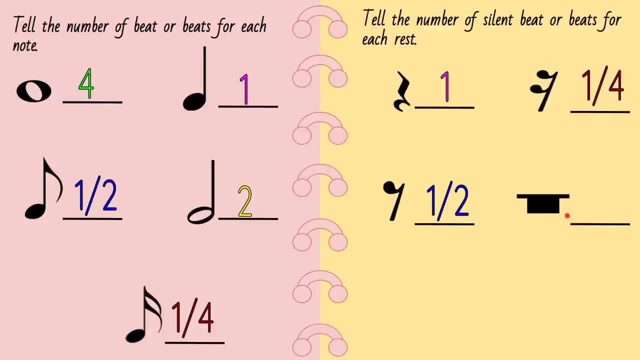 is: facing down below the line: How many silent beats Correct? It's four And this one, okay, above. facing upward: above the line: How many silent beats Correct? That is two. Okay, Let's review. Okay, Whole note. it receives four beats: Quarter note: one beat: Eighth note.